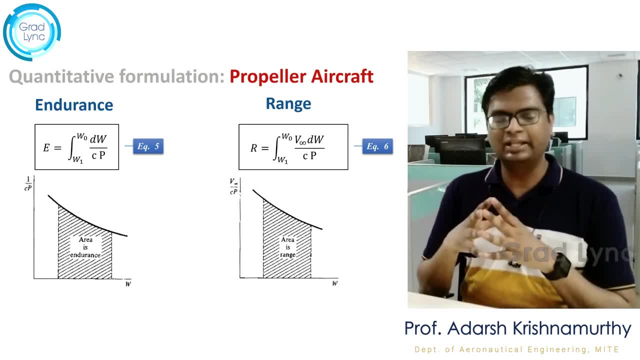 axis is 1, by Cp, The area under the curve would have given Cp given endurance for propeller aircraft. Similarly, if the y-axis is V-infinity, by C-in-to-P, the area under the curve would have given the range for propeller aircraft Clear. Then. 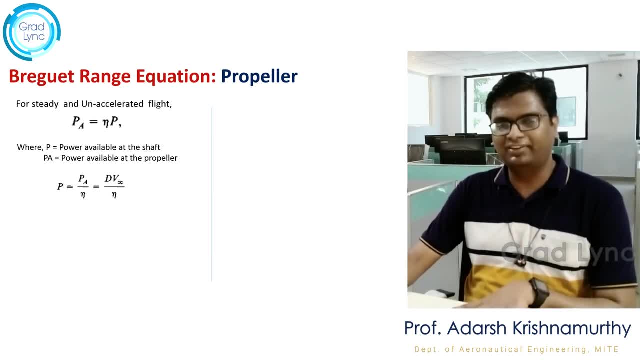 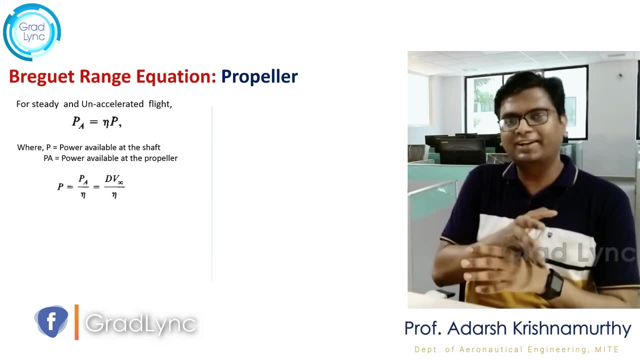 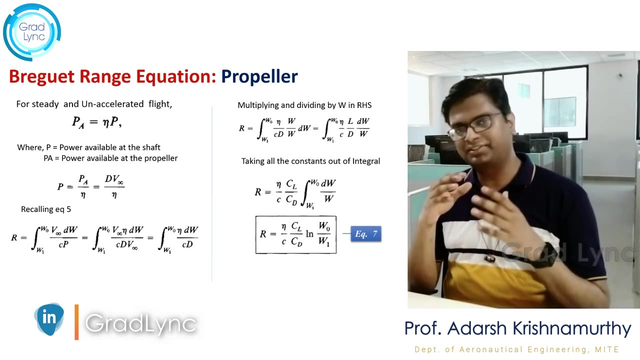 we move on to define a new parameter called as propeller efficiency, which reduces the power which is available at the shaft and the amount of power which actually gets transmitted to the propeller blades. Then we move on to derive the Breguet range equation, which 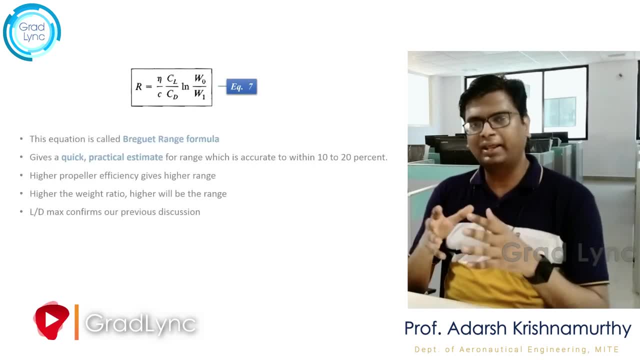 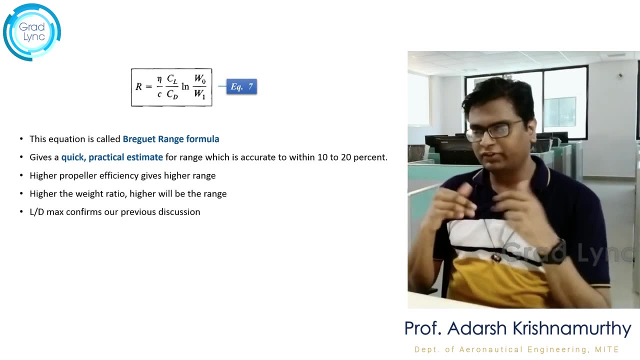 tells that for a propeller aircraft the maximum range is possible if the aircraft flies at C-l by C-d max. So we understood the Breguet range formula and various parameters it depends on. So very important in that is C-l by C-d max. 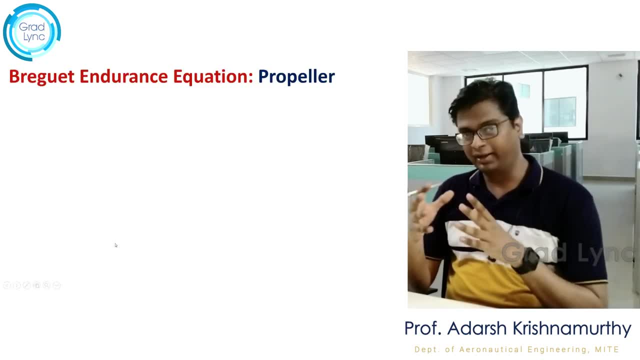 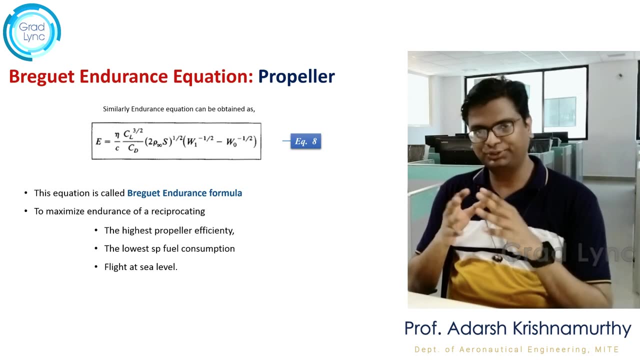 Then we move on to derive the Breguet range equation which tells that for a propeller aircraft it depends on the ciento, on D. So we understood the endurance for propeller aircraft and on what parameters it depends on, apart from all other ratios, the endurance, 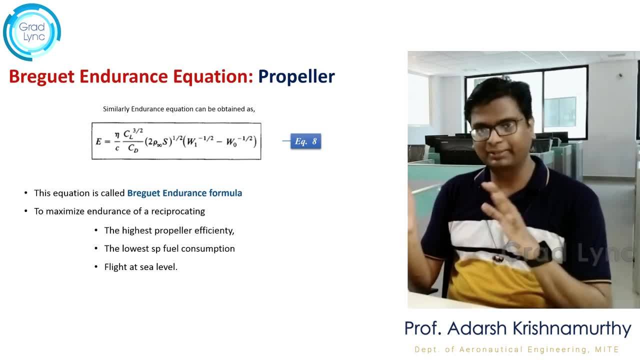 also depends on density, were, as range doesn't depends on density, So please understand few differences where, as for a propeller aircraft, you can get the maximum range C-L by C-d is max, Telling is pile performance, so its still a fairly impressive stuff. 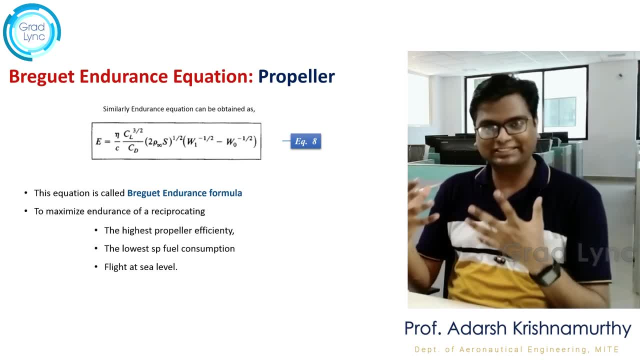 If anyяют or has any other questions related to the POC typical to you, please comment below this: maximum endurance: when CL power 3 by 2 by CD is maximum, then of course in both the cases you need to carry high amount of fuel or the rate of the fuel should be high in both the 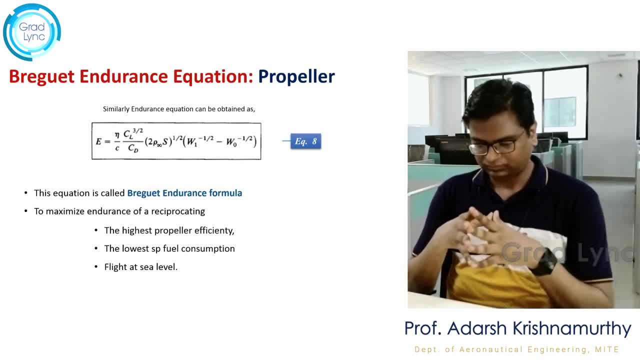 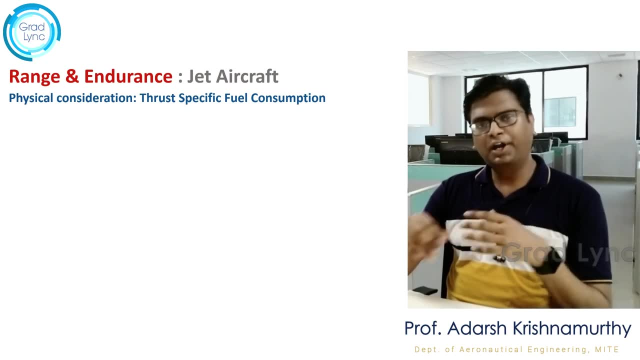 cases. right, so the same principles we will try to apply for jet aircraft as well. right? so in order to get the equations for jet powered aircraft, I need to define a new tool called as thrust- specific fuel consumption. any idea? what is the specific fuel consumption? it is 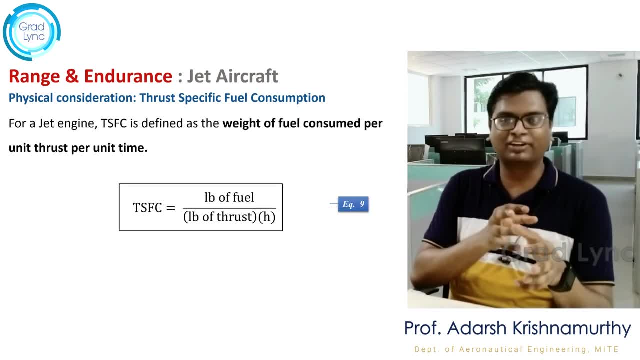 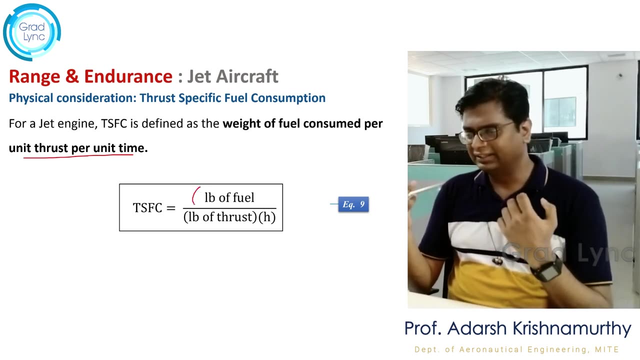 same as specific fuel consumption, but we are replacing the power with thrust. it is defined as the weight of the fuel consumed to generate unit amount of thrust per unit time. right in British units it is nothing but the pounds of fuel consumed. to the pounds of fuel consumed. 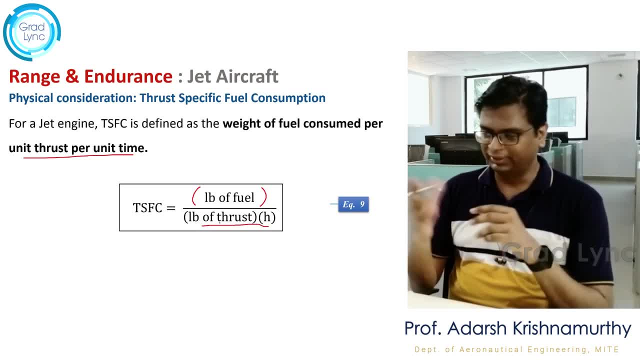 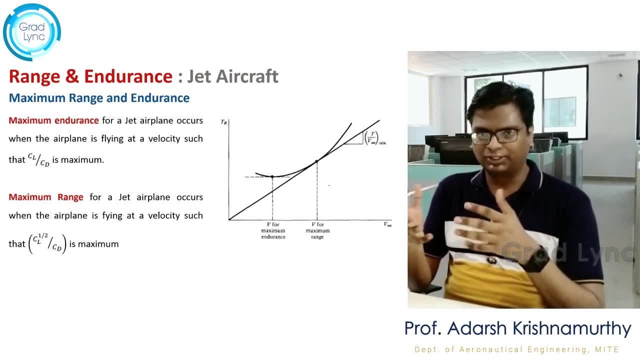 to the pounds of thrust generated in unit time. so let's call it as equation number 9. so if I draw a graph for thrust required and versus velocity, I get this particular shape where the minimum thrust required results in maximum endurance for a jet aircraft. correct and remember: for jet aircraft. now this particular curve represents the thrust required curve. 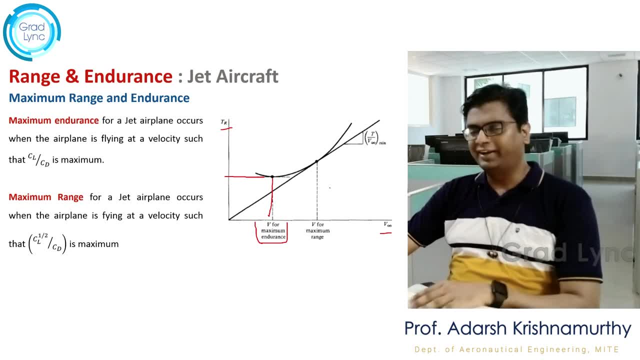 of course, and the x axis is a velocity right. it is nothing but the variation of thrust required with velocity right. so if I draw a tangent from the origin to the curve- thrust required, curve- I get a point which represents the velocity for maximum range, or in other words, that point actually. 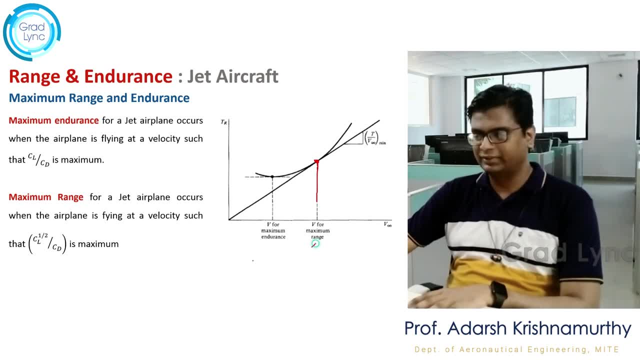 represents C L power 1 by 2 by C D max and of course the minimum thrust required condition at C L by C D max. clear getting the point so we have for maximum endurance for a jet aircraft occurs at C L by C D max, whereas the maximum range occurs at C L power 1 by 2 by C D max. 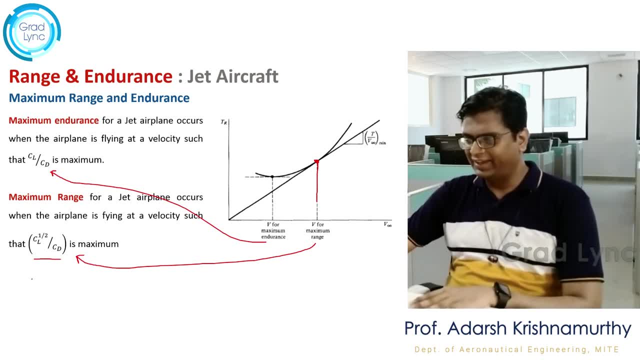 clear now, if you understand there exists a clear relationship between the velocity for maximum endurance, velocity for maximum range. You need to observe and understand one thing here: If you fly at a velocity where CL by CD is maximum, the jet aircraft is not going to achieve maximum. 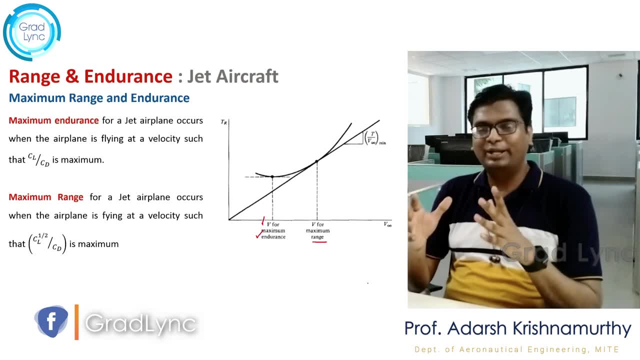 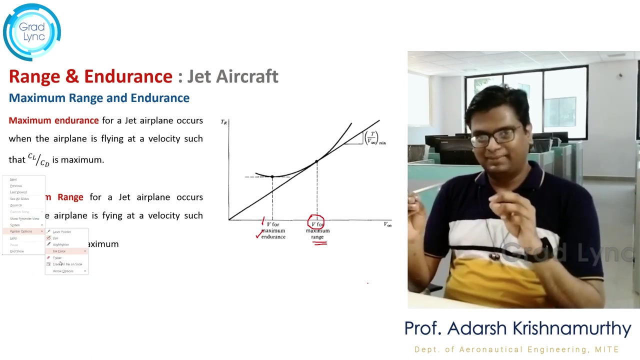 range, whereas it is going to achieve maximum endurance. But if you fly at a velocity where CL power 1 by 2, by CD, is maximum, the jet aircraft is going to achieve maximum range. understood So two important concepts you have to understand, Both maximum range and 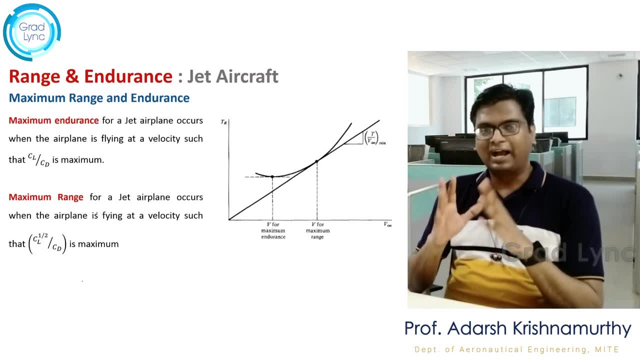 maximum endurance cannot be achieved at a given velocity. These two velocities are different, they are not same. I cannot get maximum endurance, maximum range at the same time- Not possible. If I want to get maximum range, I should fly at CL power 1 by 2, by CD max. If I need maximum endurance, I should 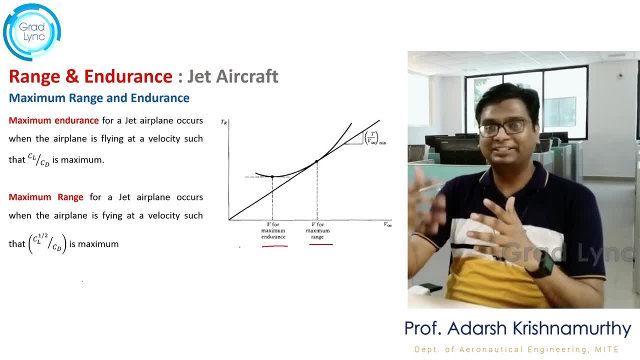 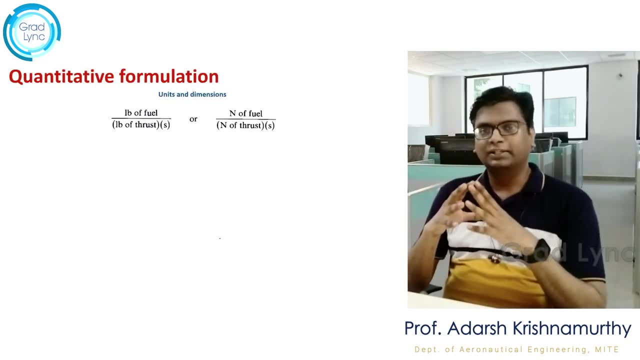 change the velocity of my aircraft such that CL by CD is maximum. Next we'll try to understand the units and dimensions of the thrust specific fuel consumption right. So the unit of thrust specific fuel consumption in MKS is pounds of fuel per pounds of thrust generated multiplied by seconds, that is, per unit time, Or in SI unit. 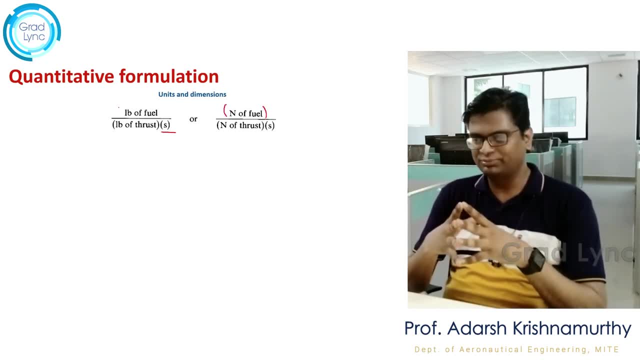 you can represent it as the Newton of fuel consumed to the Newton of thrust generated, multiplied by time. right Now, in order to continue the analysis, I am going to introduce any new product called as the thrust specific fuel consumption, CT, multiplied by the thrust available and multiplied by the time increment. So this product is going to give me the 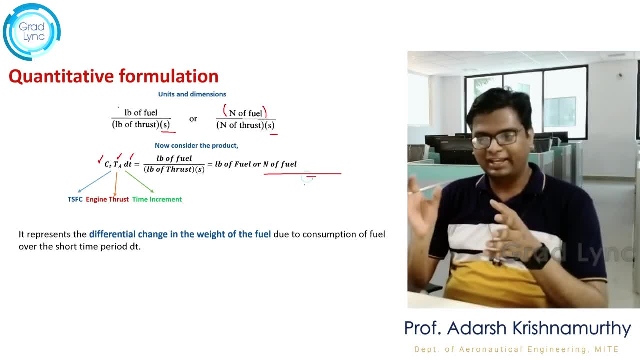 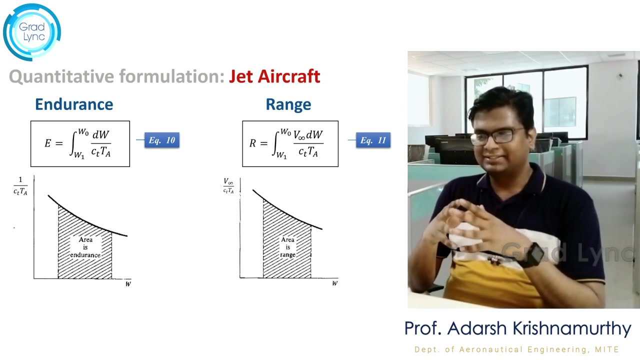 Newton's of fuel getting consumed in a time. DT right. It represents the differential change in weight of the fuel due to consumption of the fuel over a short period of time. DT Now. with the same analysis, I got the fundamental equation for range and endurance for a jet aircraft. as for endurance, I have the integral from W 1 to W 0. 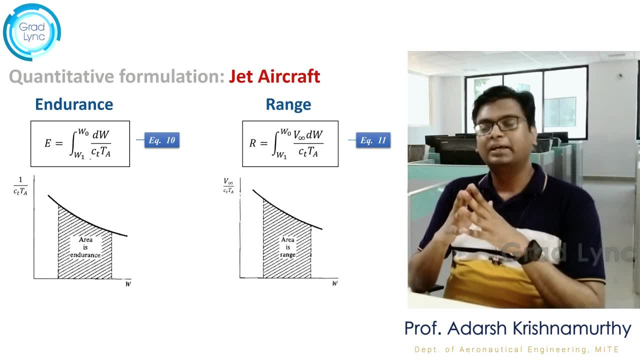 DW divided by CT into T a, Where CT is the thrust specific fuel consumption and T a is the thrust availableу clear, Let's call this as equation number ten And if I try to represent that in teller, helix Is the thrust possible. 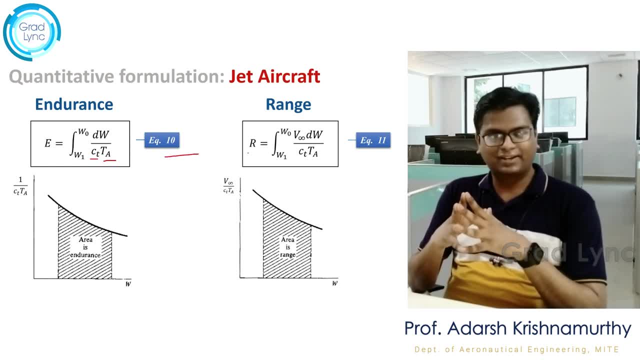 10.. I can see just by looking at the explanation information all the equipment does fine in these. this in a graph of 1 by CT into TA versus weight of the aircraft. The area under this curve represents the endurance for a jet engine aircraft. Similarly for range I can obtain: 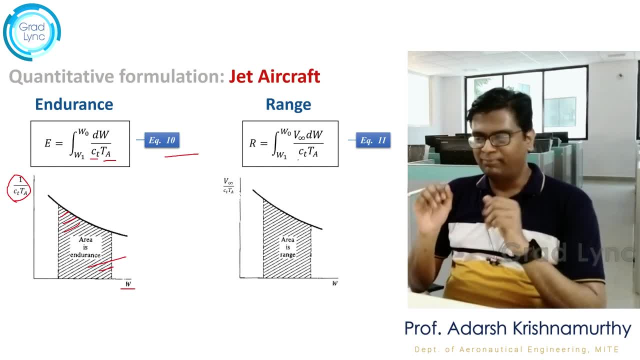 an expression which is equal to the integral of W1 to W0, multiplied by integral of W1 to W0 of V, infinity by CT into TA, into DW, right, Let's call this as equation number 11.. And if I draw a graph, V infinity by CT into TA versus W, the area under this graph represents: 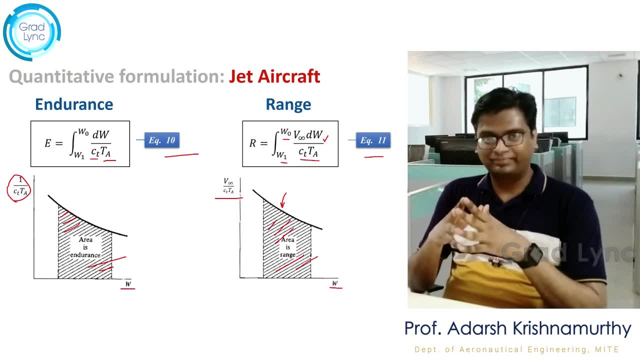 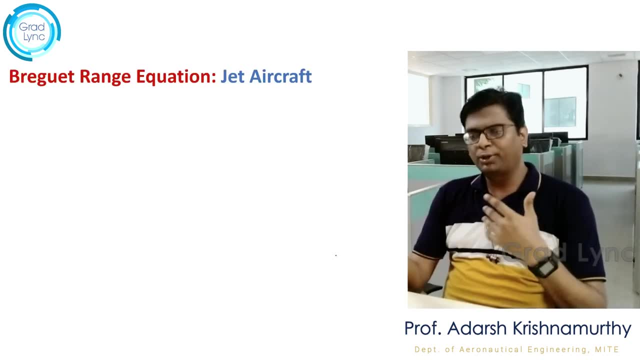 the range of a jet propelled aircraft. Let's move on to derive the Breguet range equation for a jet aircraft. I am not going to discuss the derivation here. You can refer aircraft performance and design by Anderson. for that The procedure is same as for propeller aircraft. Right, you have. 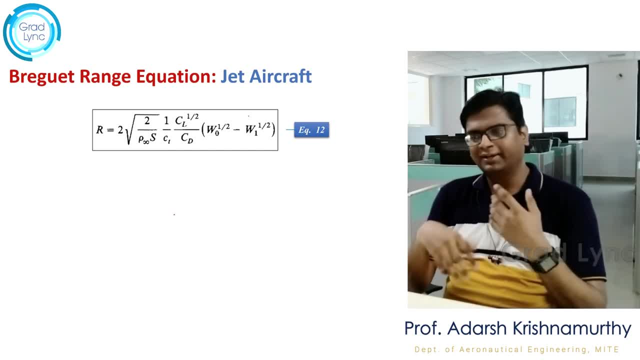 to replace the specific fuel consumption by thrust. specific fuel consumption, Right? so, finally, I am more interested in understanding the range equation rather than getting at the equation. Getting at the equation: the methodology is same. there is no change, right? So let's try to understand this equation, and I am calling that equation as equation number 12.. 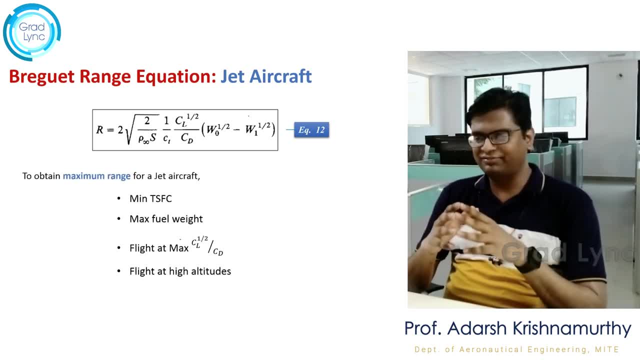 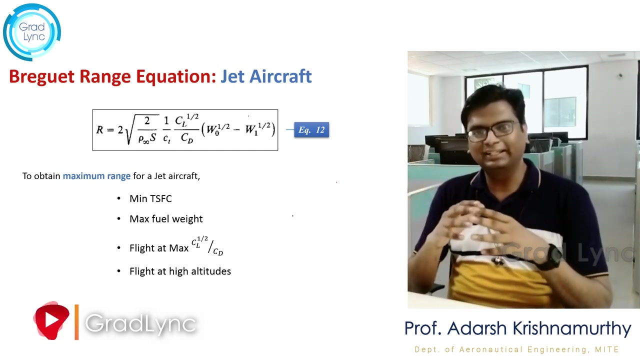 So you can obtain the maximum range for a jet aircraft when the thrust specific fuel consumption is minimum. Of course, this is one obvious observation you can make for all the four equations, that is, range and endurance for jet and propeller aircraft. Minimum fuel consumption or thrust specific fuel consumption results in maximum range, maximum endurance, more range and endurance for jet engine as well as for propeller engine aircraft. 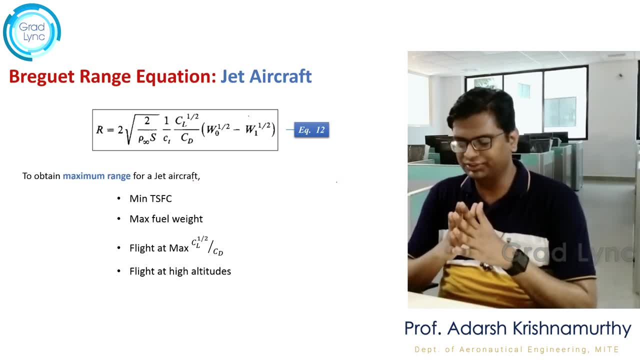 Clear. So this one point is common in all the four equations. Then of course, I have maximum fuel weight. This is also a common trait in all the four equations. If you carry more fuel, you can cover more range and endurance will be more. 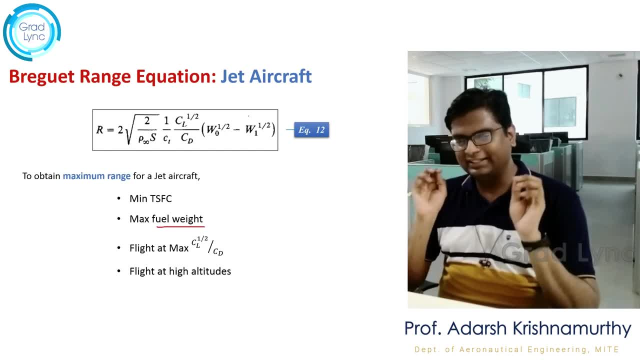 Clear. But the important changes comes here. What is that? The ratio of coefficient of lift to coefficient of drag. So for maximum range for a jet engineer craft you should fly at CL power 1 by 2 by CD max. Right Just now we saw the graph how we can achieve that. 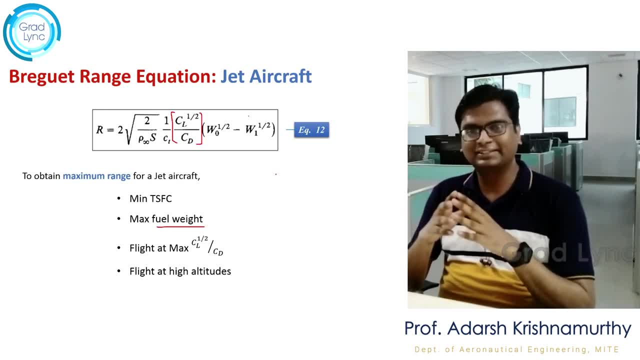 Understood. So CL power: 1 by 2.. 2 by 2 by CD max gives the aircraft maximum range. if it is a jet aircraft, and also if the aircraft flies at higher altitude, range will be high because here in this equation the density is inversely proportional to range. as the altitude increases, density is going to reduce and range is going to increase. 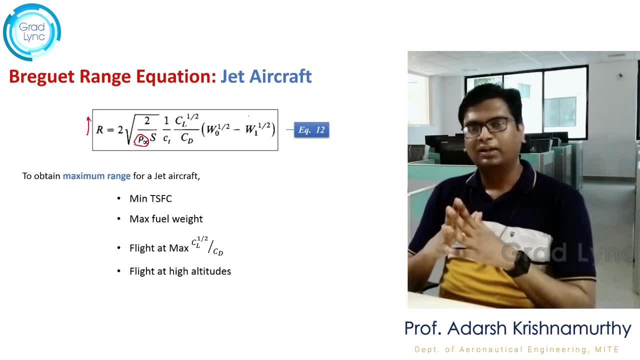 That is the reason why. That is the reason why Turbofan engines are used for intercontinental travel And propeller aircrafts are used for local travel, let's say, between New Delhi and Mumbai. They may use the propeller aircraft, which gives a better efficiency at lower altitudes. 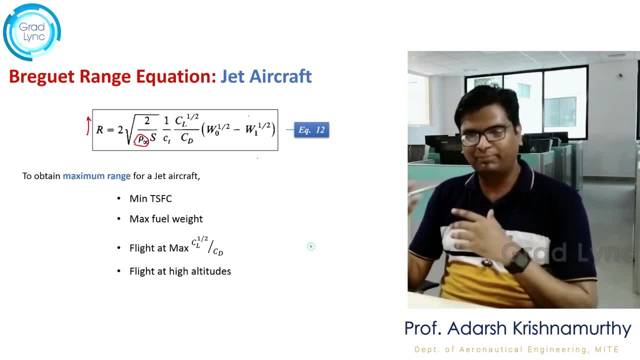 Whereas if I want to travel to New York from Delhi, so I would prefer to buy a turbofan engine aircraft rather than a jet aircraft. So I would prefer to buy a turbofan engine aircraft rather than a jet aircraft, propeller aircraft, because the distance is more so I want to travel at higher altitudes. 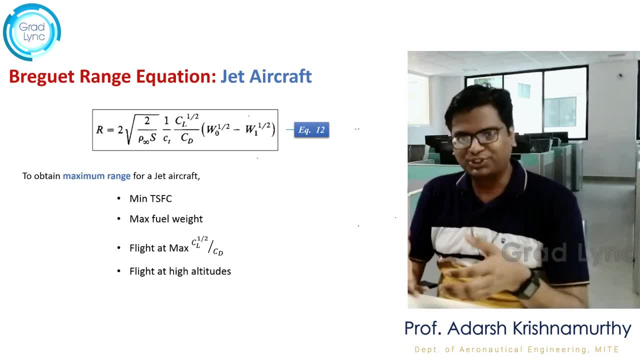 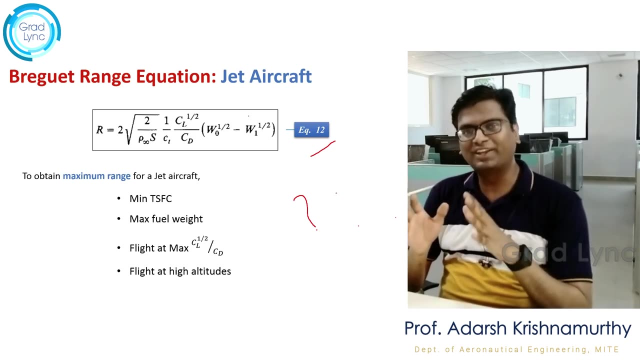 to reduce the fuel consumption. so this question has been asked in many interviews: why or what is your preference of aircraft for intercontinental travel? right, so many of them can answer this question, but you should know the reason behind the answer, right? so this is the reason. the range is inversely proportional to density, so as the altitude increases density. 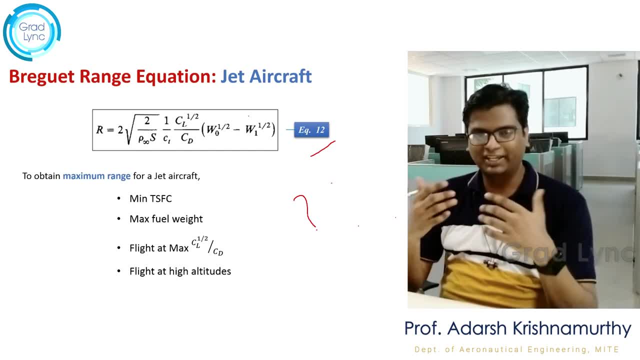 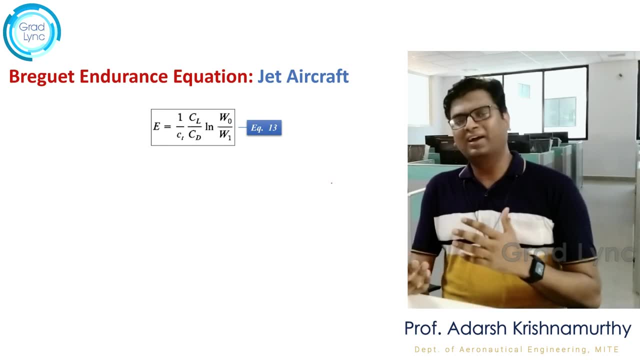 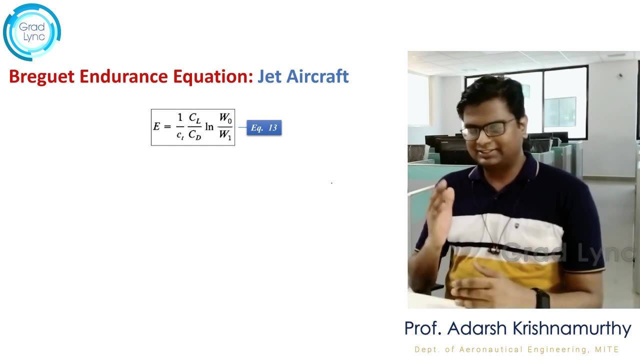 is going to reduce. as density reduces, range is going to increase. let's move on to the endurance equation. I got the endurance equation as the same as I got for propeller aircraft. endurance is given by 1 by ct. that is the thrust: specific fuel consumption multiplied by cl, by cd, into natural. 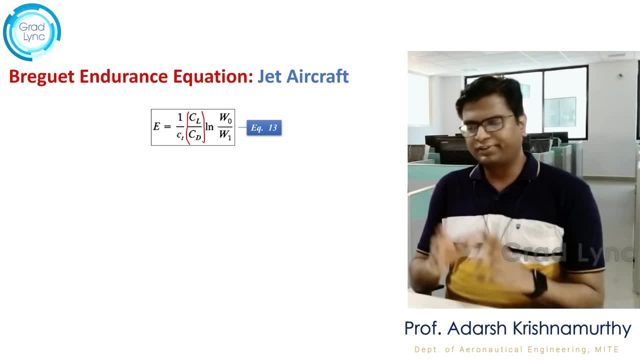 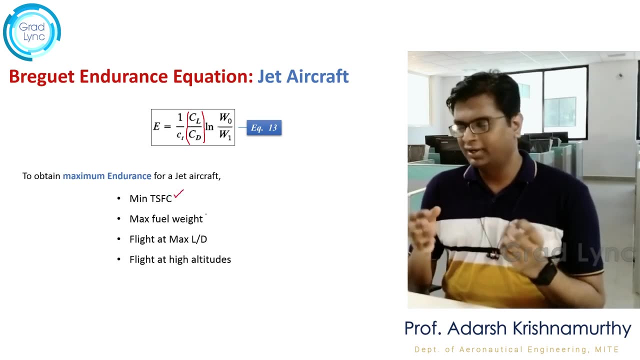 logarithm of d. so you observe carefully, apart from all other parameters. that is, if you fly at minimum thrust, specific fuel consumption, definitely the endurance is going to increase. apart from that, the point you should understand here is if the aircraft flies at cl by cd max, right then it is going to get.